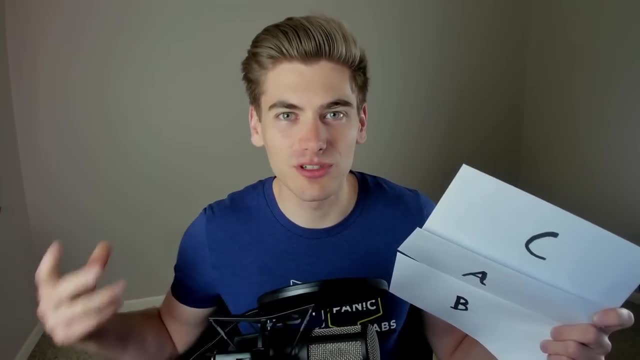 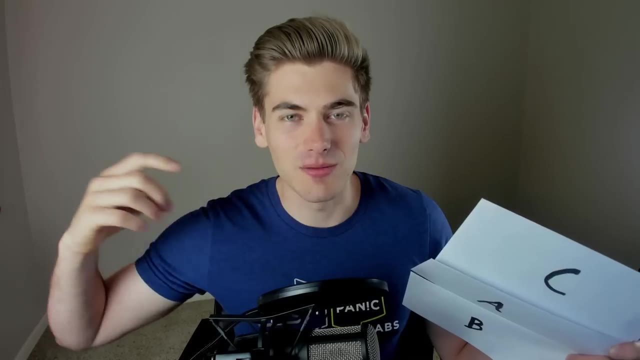 when you're writing out code and you need to understand what your code is doing and how it's going to perform with the data that you're given. all of these different thought considerations around speed and memory usage are what big o notation is built around and the idea of big 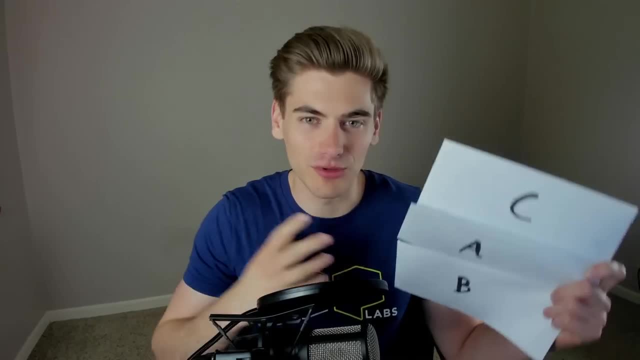 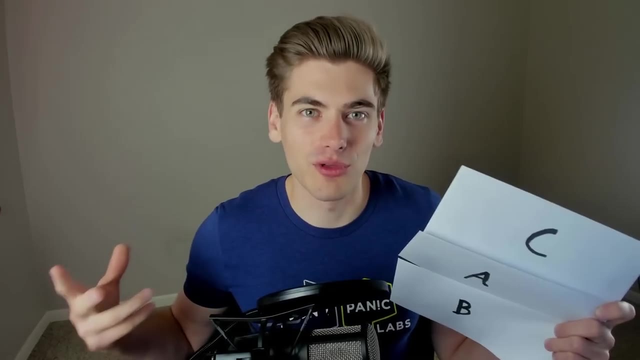 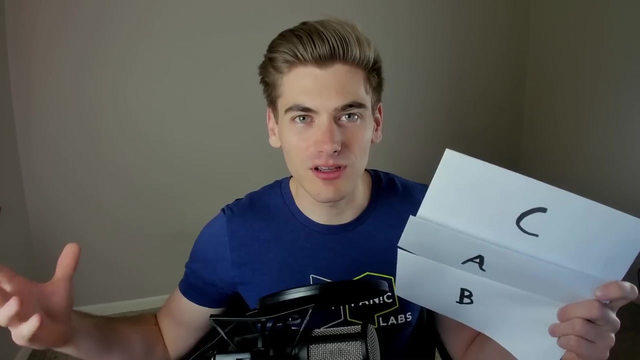 o notation is analyzing the algorithm you create, for example the sorting algorithm for these letters, and figuring out how much space does this take up or how long does this algorithm take as the size of my input changes. so as i get more and more letters, from 3 to 30 to 300, will my algorithm take? 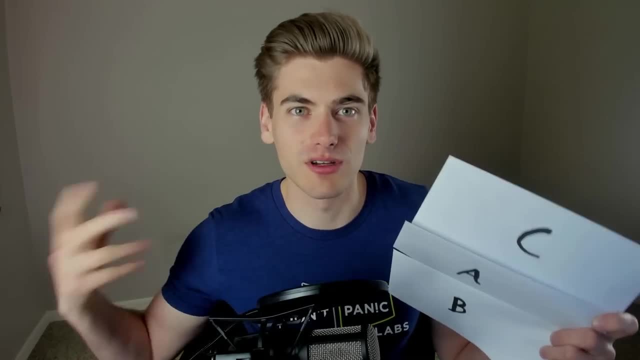 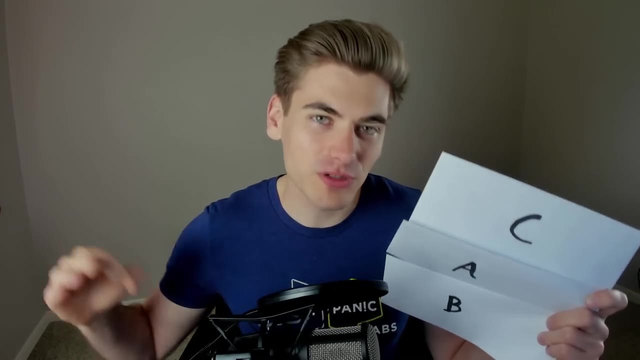 up more space, or will it become slower and slower and slower. and not just will it become slower or will it take up more space, but how much slower will it get and how much more space will it take up compared to other similar algorithms based on the same? 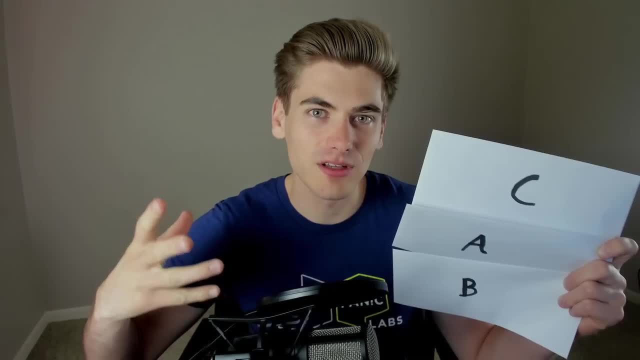 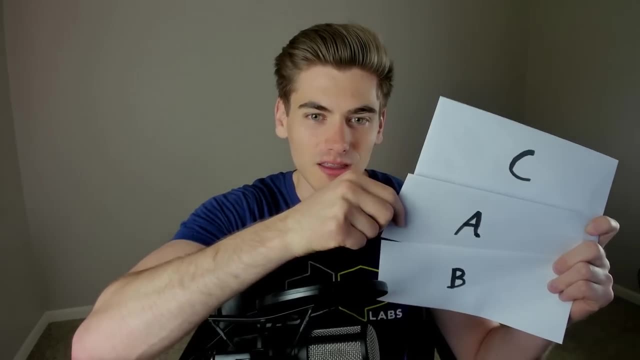 sets of inputs. so you can imagine that we have these letters and there's a few different ways i can sort them. for example, i could go through and find the smallest one. for example, a is going to be first and i could take that and put it into a new list over here. then i could go through and i 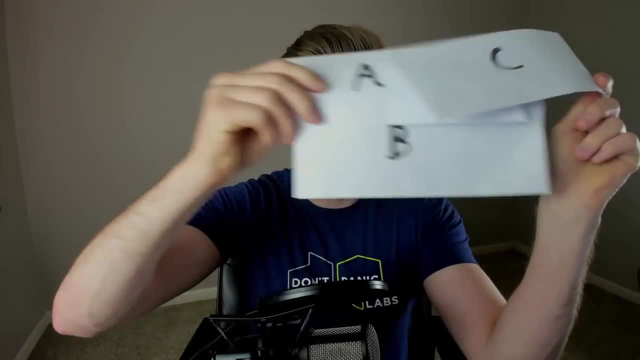 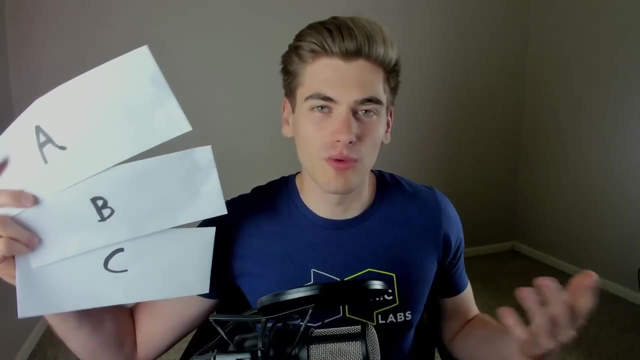 see b down here at the bottom, and i could put that after a, because that's the next one in the list. i could go in and i could take c and i could slot that in at the very bottom of the list. and there we go. we have a sorting algorithm and while it's not the quickest algorithm in the world, 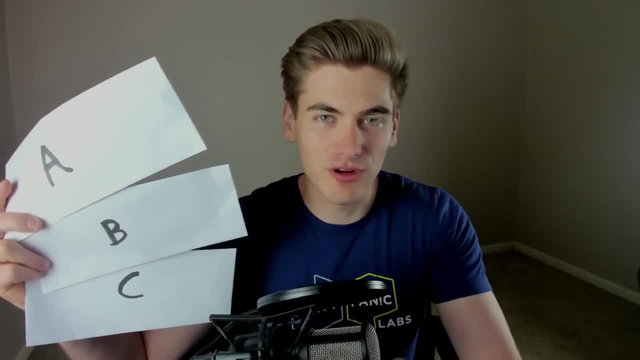 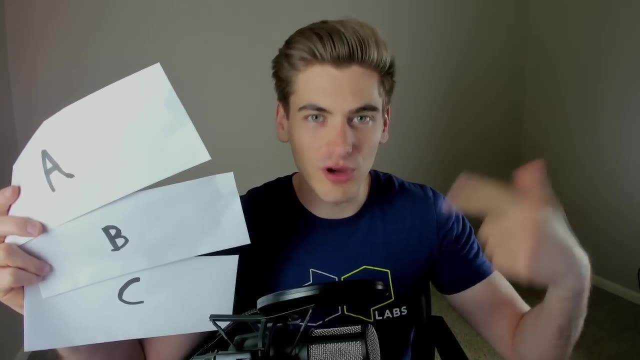 it gets the job done. but you noticed, we took up two different arrays. we had a list over here in my right hand and a list in my left hand, so we had double the space and we had to loop through our first list over and over and over again, which is not that quick. so this is just one example of a 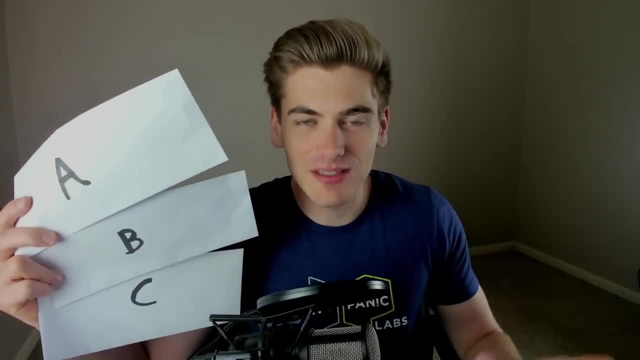 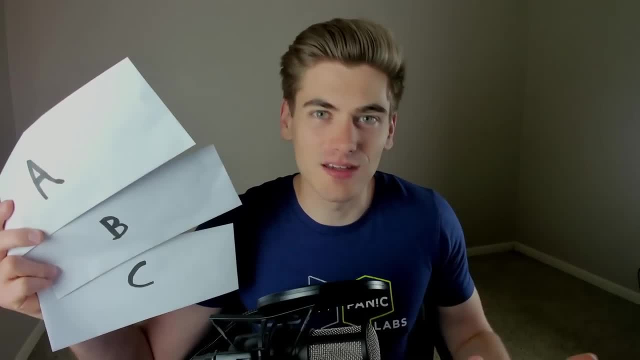 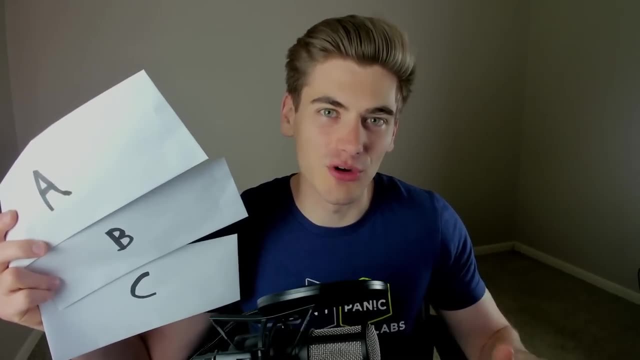 abstract examples of envelopes in my hand and trying to turn that into code. so let's jump into the code and actually look at some simple examples to figure out how you can analyze them and determine their big o notation. so here we are with a really basic example where i have an array right 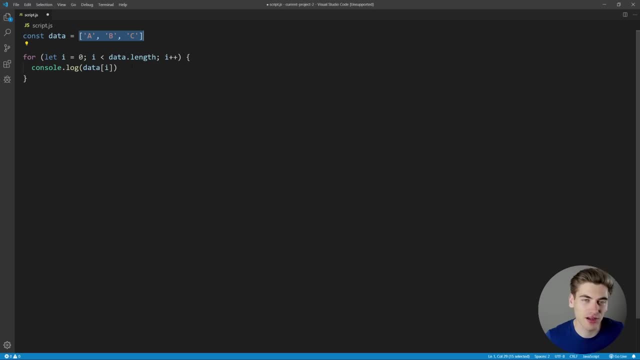 here of data, three long, and we're just looping through and console logging all of the elements in our array, one after another, and for our purposes of this algorithm, which is this for loop. here we want to determine how slow this algorithm is, essentially as our input grows. we want to 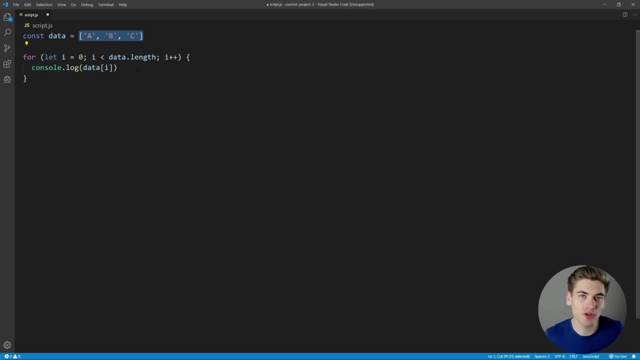 determine how slow this algorithm is, essentially as our input grows. so, if we go from three to 300 inputs, how much longer is our algorithm going to take? how does it scale as our input scales? so, generally, when you're doing these kinds of determinations, the first thing you need to do is: 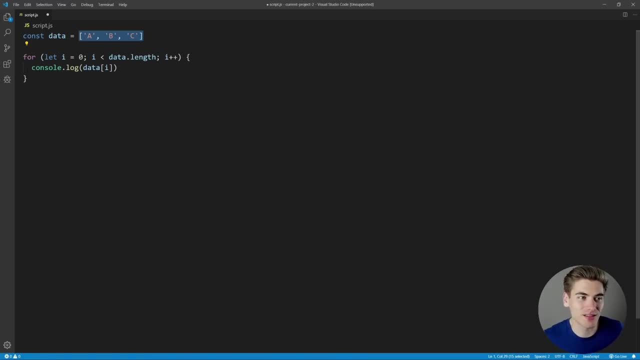 figure out what the core part of your algorithm is. in our case, this core portion is this consolelog. it is the one thing that our algorithm does over and, over and over again to get the end result. and then we take this and we determine how many times does this thing happen, based on how large our 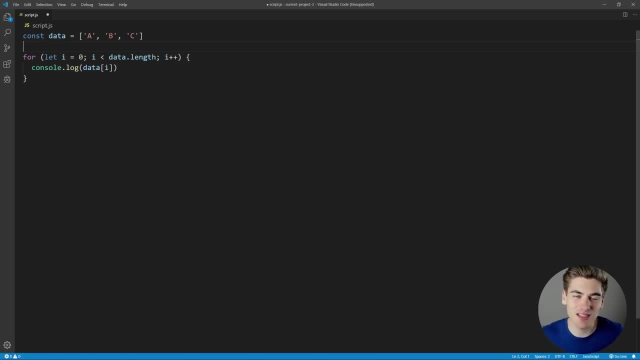 input is, and then we take this and we determine how many times does this thing happen, based on how large our input is. so, generally, what you're going to do is you're going to set some form of variable to be how long your input is. this is almost always used as n, so you'll see n a lot in big o notation. so 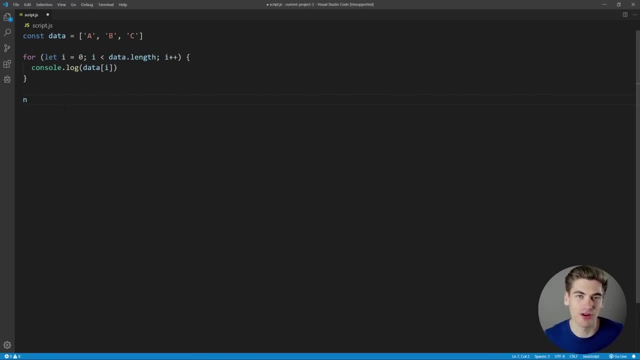 we'll say the length of our data array is equal to n in our case, and now we want to determine how our algorithm grows as n grows and, in our case, as n goes from 3 to 300. we run this loop three times and then 300 times, so it scales one to one with the size of n. so we would give this a. 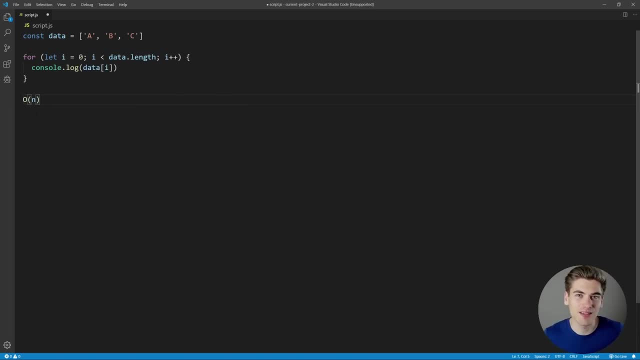 big o notation of n. we'd say big o of n- is how this algorithm scales with the size of our input, based on time. so as our input scales from 3 to 300, our algorithm is going to scale in time linearly. essentially it's going to grow one to one with the size of our input. if we were to, for example, do: 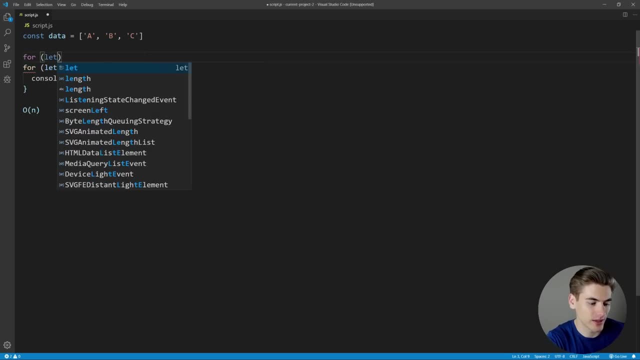 another form of loop. we put a loop outside of here. we'll say, let say j equal zero, j is going to be less than data two. oops, two dot zero. so we're going to put a loop outside of here. we'll say: let length, and then j plus plus. and now what we do is we consolelog out data 2 of j. 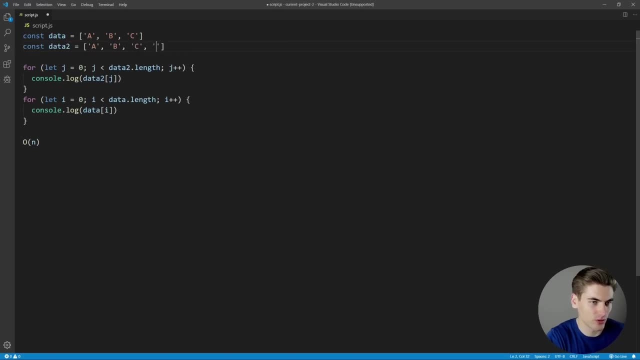 and let's just create data 2 right here and we'll give it, you know, one more. we'll say actually: oops, data 2 is going to be 1, 2, 3, 4 or 5.. so now what we have is we have two different loops in. 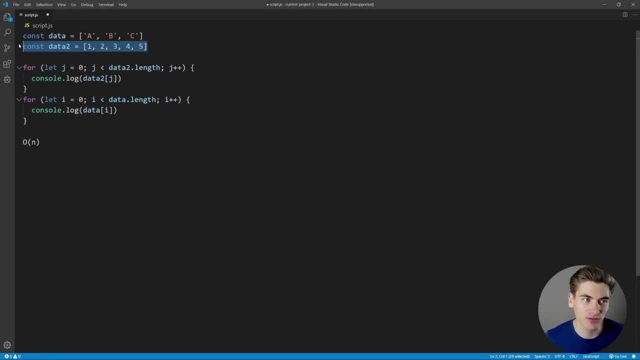 our algorithm. our algorithm first loops over everything in data 2, right here, and then loops through everything inside the data 1.. so now we have two separate variables. we have n, which we're going to use for our data 1, and then data 2. we need to come up with some other variable. 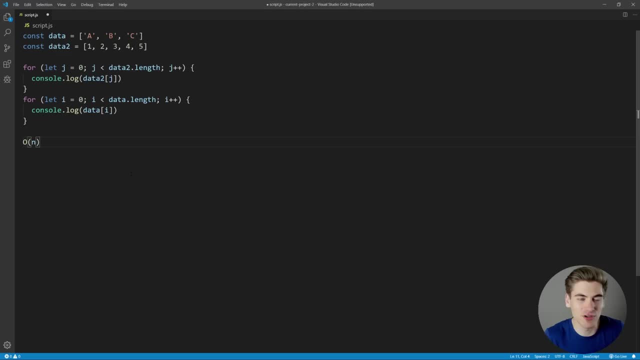 we can just say, for example, b. it really doesn't matter, we could just even do a and b, but in our case we'll have n represent data and b represent the length of data 2.. so now our algorithm is going to scale based on the length of data 1 and data 2.. so we have a big o here of n plus a, because 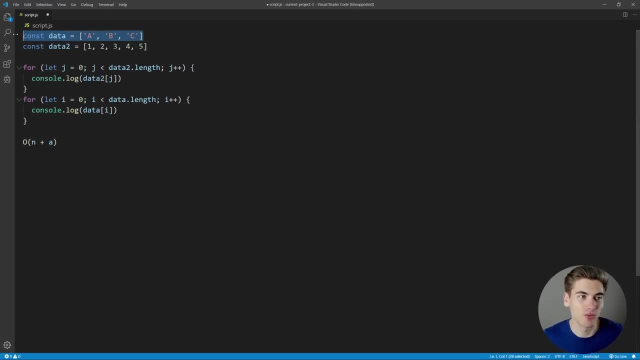 we have data 2, which is a, that's the length of data 2, and data 1, which is the length n, and we're scaling off of both of those because we loop through everything in data 2 once that's a. then we loop through everything in data 1 here n times because that's the length of our array. 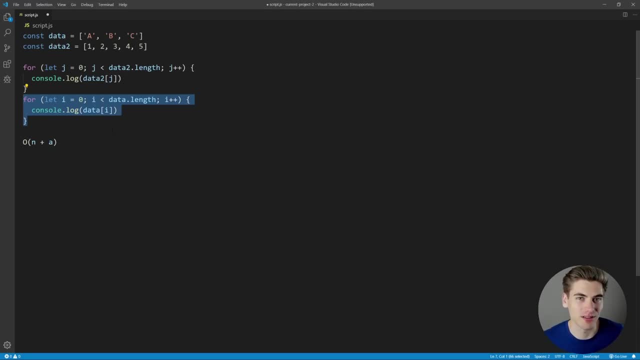 so we have an n plus a length loop here, as you can see. if we were to modify this slightly, though, and that we have our loops inside of each other, so if we come down here and we want to say, for each one of these, what we want to do is, we want to log data, and then we also want to log here, data 2. 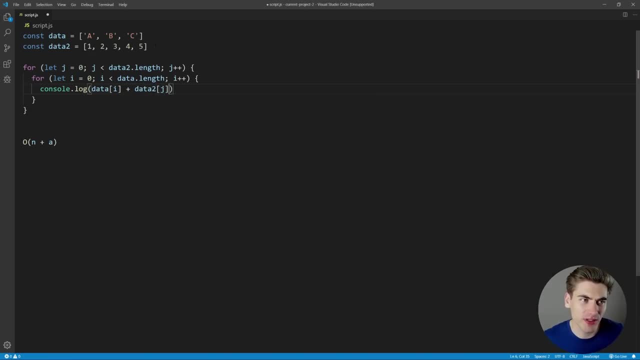 of j. so now we're looping through every single element in data 2 and then for each one of those elements we're looping through every single element inside of data 1.. so now we have nested loops and now our big o notation here is going to be right, here our 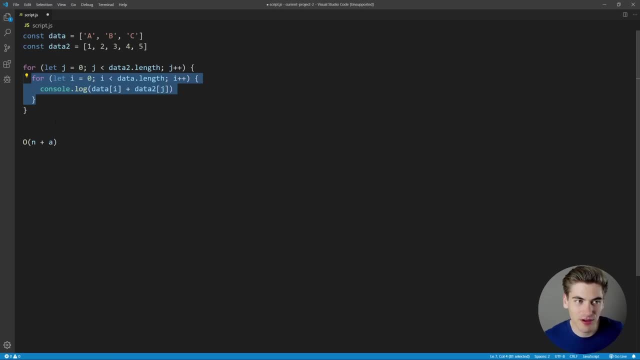 console log 1 and we're doing this n times here for every single a time that we go through our loop. so this is actually n times a as our big o notation to represent how long this algorithm takes, because if we add 1 to our a element here, so we go from 5 to 6. now this is going to be. 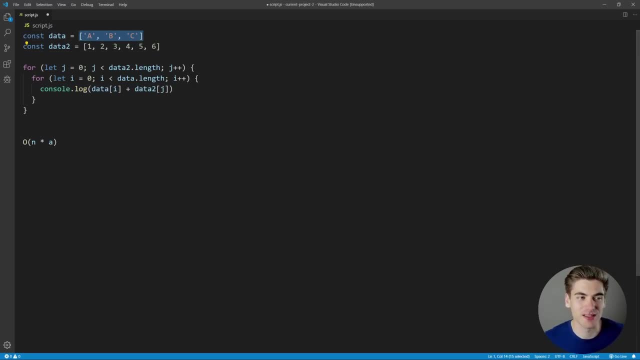 looping through our algorithm one more time and then we're going to be looping through data 1 time for each element inside of our data here because we have these nested loops inside of each other and generally when you start seeing nested loops like this, you're going to run into 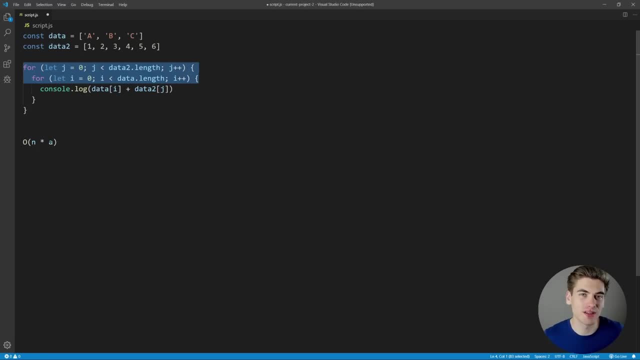 pretty poor performing algorithms and your big o notation is going to scale quite quickly. for example, if we just simplify this and make this data here, get rid of data 2 completely and we're just going to print out data of i and data of j, just like this, that would be essentially 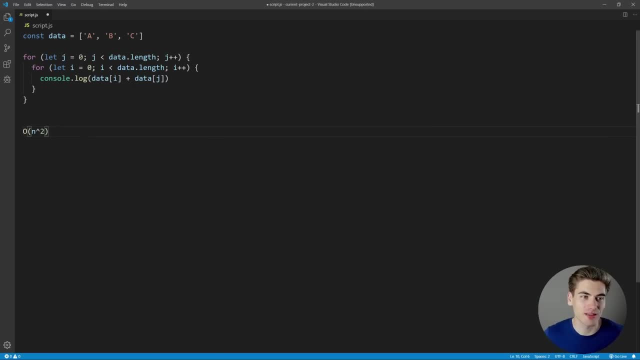 n squared over here for our big o notation, and that's because every single time we loop through n, we have to loop through n again for each element of n. and when you start to see these types of algorithms, this is when you start to run into problems, because these perform very 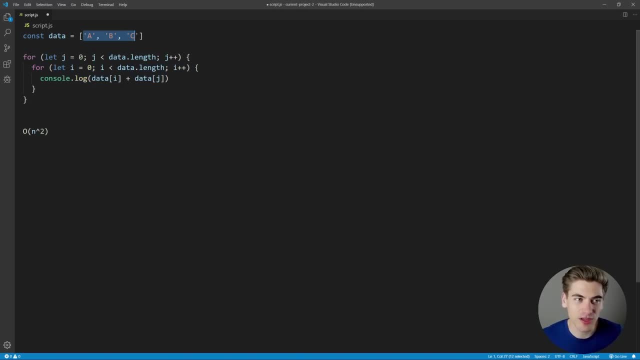 slowly as your input grows. for example, with an input size of 3, we perform this console log 9 times. but if we just bump this up to 5 now we have to perform that 25 times. so it's growing exponentially and you'll see it just skyrocket off. if your input is 100 long, you're going to 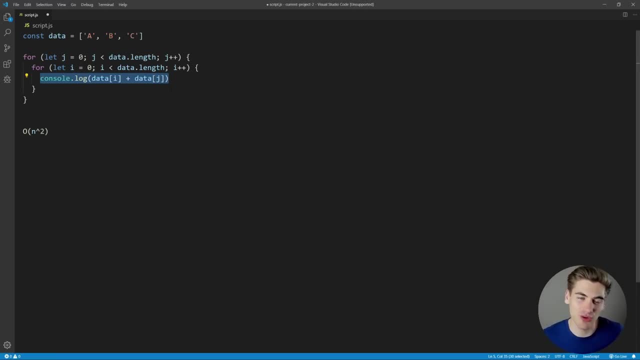 have to perform this inner part tons and tons of times and it's going to really slow down your algorithm. now what if we take this and instead of having this one console log, we do this four times? for example, you, you would think this would go to four n squared, but when you're doing big o. 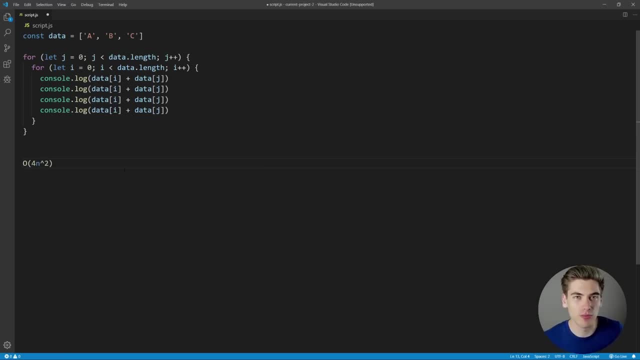 notation. one thing that you almost always are going to do is remove any leading constants like this. so this four, we don't really care that it's four n squared, because the four is kind of meaningless. it's just based on the size of the input here. what we really care about is this: 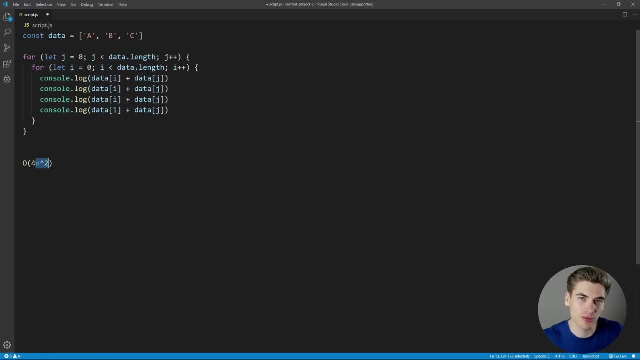 n squared here. this is really going to tell us how the algorithm grows over time, so we can just completely remove any leading constants like this. or if we even had like a plus 2 here because we logged out before our thing started twice, we can remove that as well, because 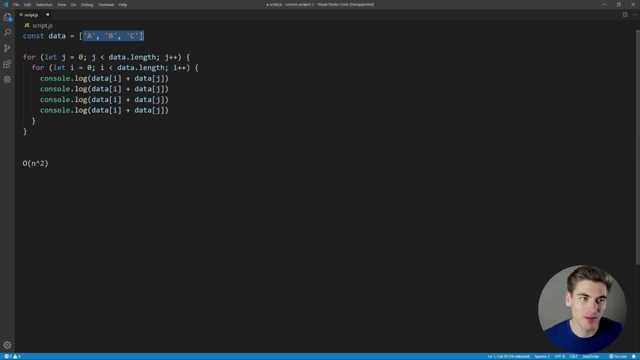 we only really care about how it grows over time based on our input. so any extra constants or any extra added numbers like that we can just completely remove. and again, speaking of extra added sections, let's say we took another loop and added it down here where we looped. 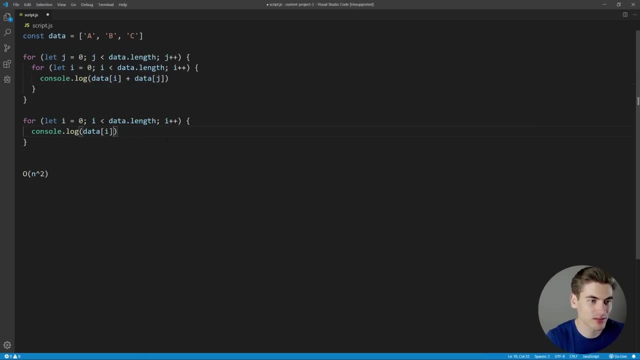 through each one of our elements again. we just printed them out like this. so now we have a, our console log here and our console log here. so this is n squared plus n, because we're looping through n squared times here and n times here. but when you see this kind of scenario, we just cut off. 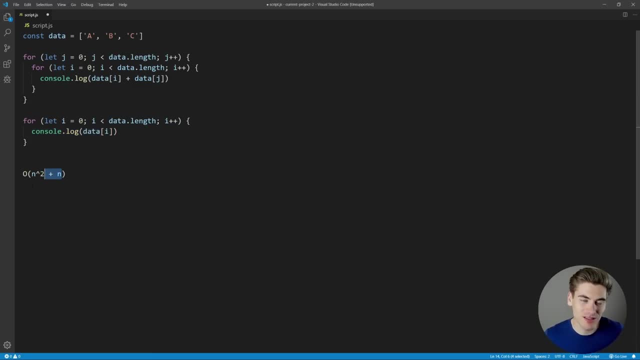 all of the things that scale less. so n squared scales way quicker than n, because 4n squared is going to be 16 and obviously 4 for n is just 4.. and as n grows in size, n squared is going to grow way quicker than n. so we just delete the n. we don't care about the things that. 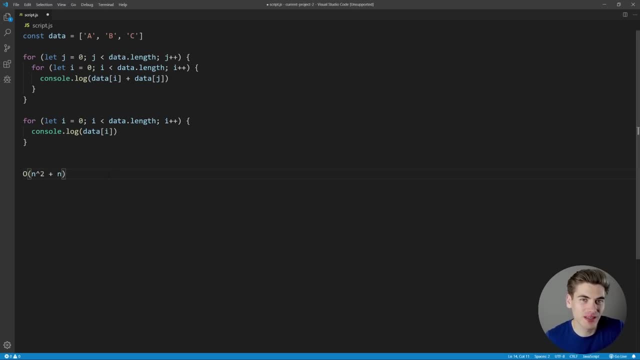 scale less quickly. now, for the most part, we've only been looking at time-based big o notation, but another way you can look at big o notation is based on space complexity. so how does your algorithm grow in memory usage as the input size scales? so let's just delete all of this that we 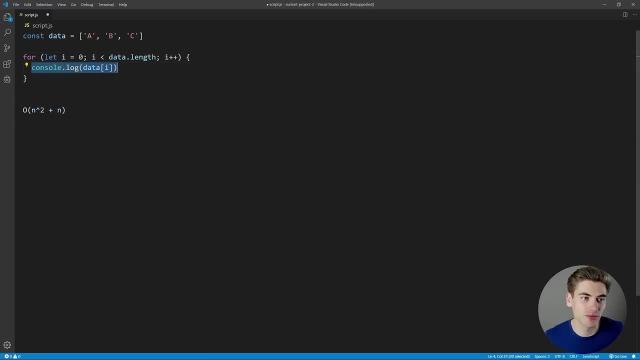 have up here and let's just be left with this basic for loop that we started with, and you can see that our space complexity for this is essentially zero. we're not adding any extra space because we're not creating anything inside of this, so you would call that essentially a big 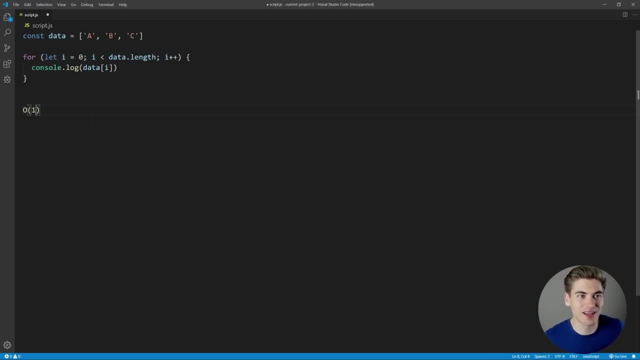 o of one, because it's going to be constant. the space does not change as our input size scales, because we're not actually creating anything inside of this. but what happens if we were to create a brand new array? let's say we come out here, const out it's going to be equal to an array and inside 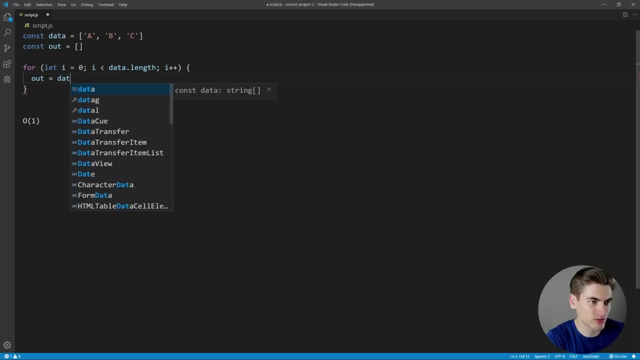 of here. we're just saying out is going to be equal to data of i and we want this to be out of i. there we go. so now what we're doing is we're creating a brand new array, essentially from the values inside of our data array. 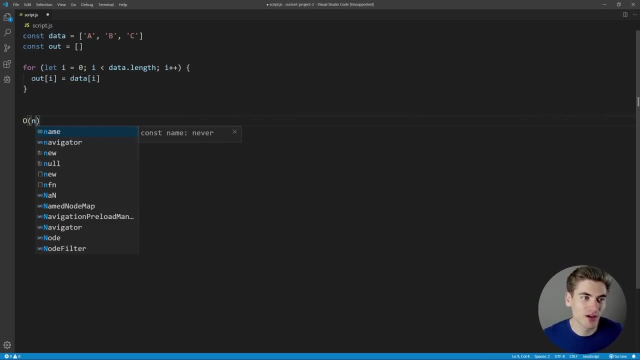 and this is going to be a space complexity of n, because our output is going to be the exact same length as our input. here. they're both going to be a length of three and the amount of memory that this algorithm takes up is exactly the same amount as the input size of our element. 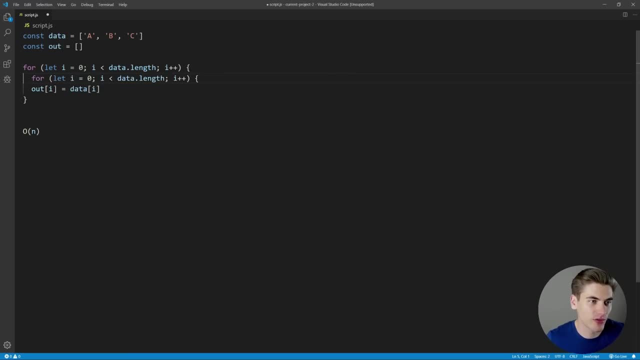 but if we were to go even a step further and let's say we created another for loop inside of here based on j, we'll do j plus plus, and here we created a brand new array. so we have out oops, out of i is going to be equal to a new array, and then the out of i of j is going to be equal to this. 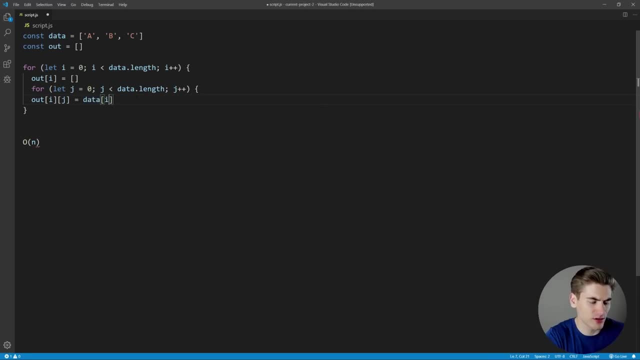 data of i, in our case actually j. data of, yeah, data of i. so what this is going to do is this going to output to us three new arrays inside of our output, and the first array is going to be the letter a repeated three times, b repeated three times, and then c repeated three times, and this